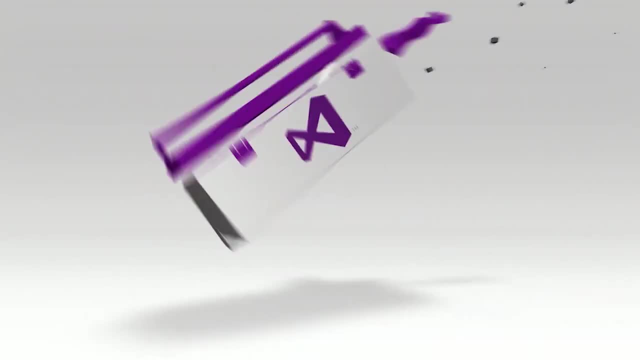 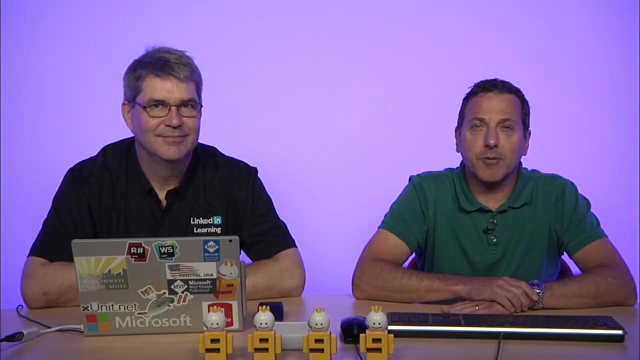 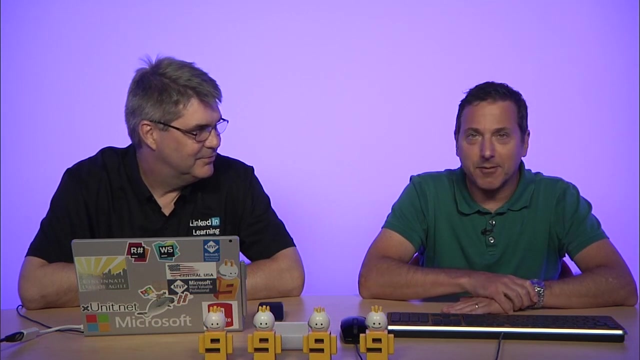 Hi, welcome to Visual Studio Toolbox. I'm your host, Robert Green, and with me is Phil Gepixy. Hey Robert, Hey Phil, How are you Good? This is the last of our design pattern series. Well, the last that we're recording in this marathon. 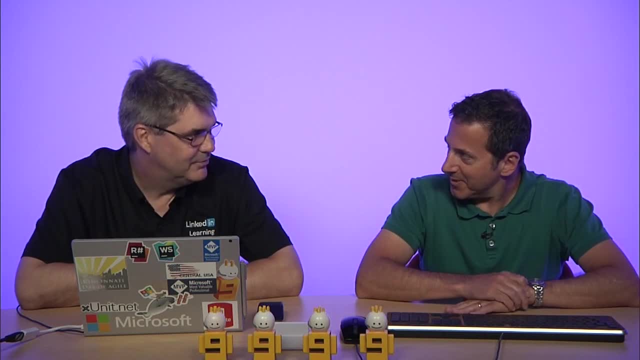 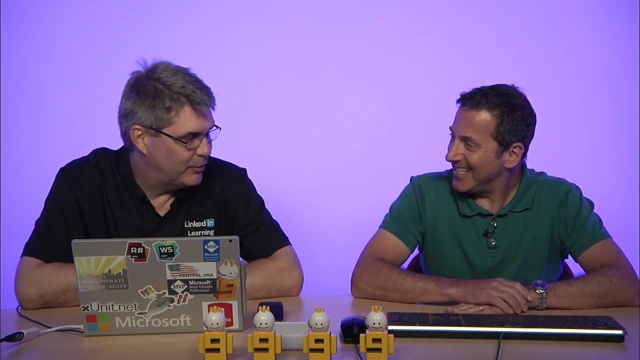 Yes, We've been in the studio yesterday and today. This is our ninth episode over the two days By the time we publish this. who knows, there may be more. There are plenty of design patterns out there we haven't covered. Yeah. 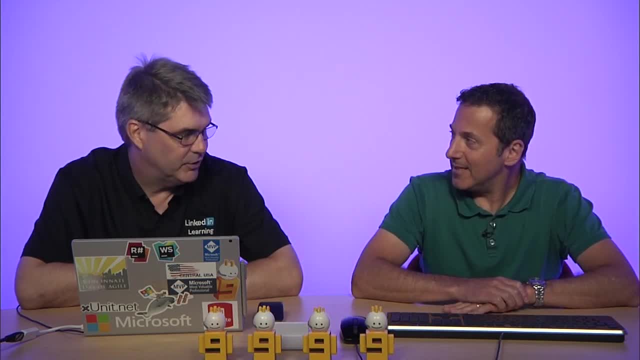 So we'll go back to the drawing board and if we get a lot of requests for a specific pattern in the show notes or in the comments, then we'll come back and do more Cool. So we're going to cover the decorator pattern today. 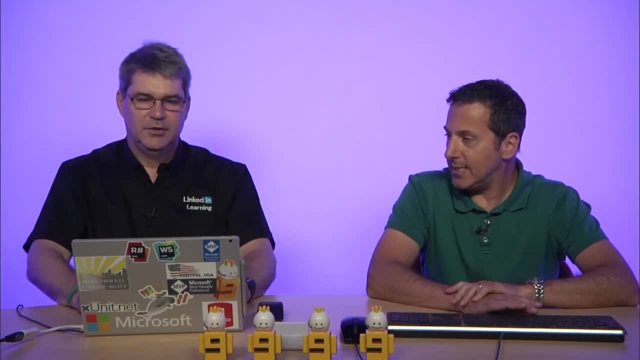 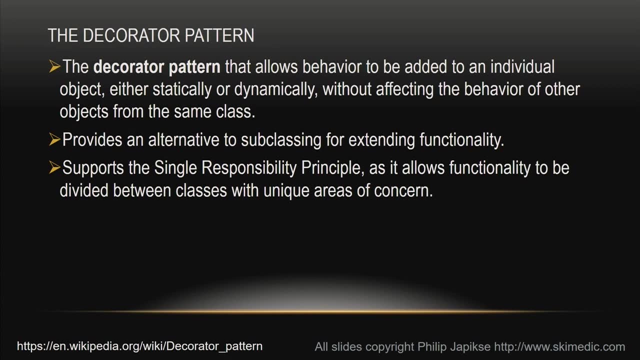 Correct. All right, What is that? So let's go back to Wikipedia for the definition. The decorator pattern, according to the official definition, allows behavior to be added to an object without affecting the behavior of other objects of the same class. Okay, In a lot of words. 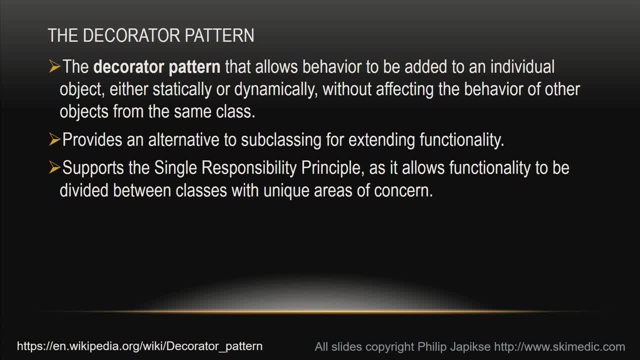 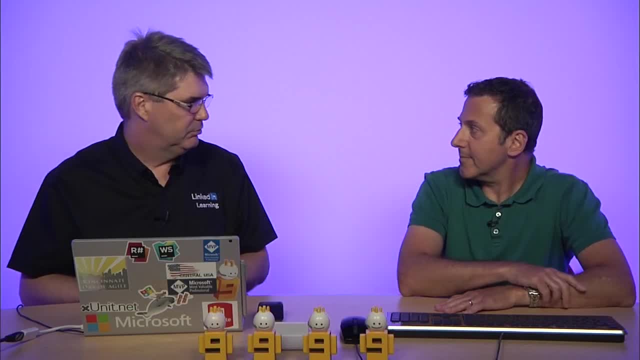 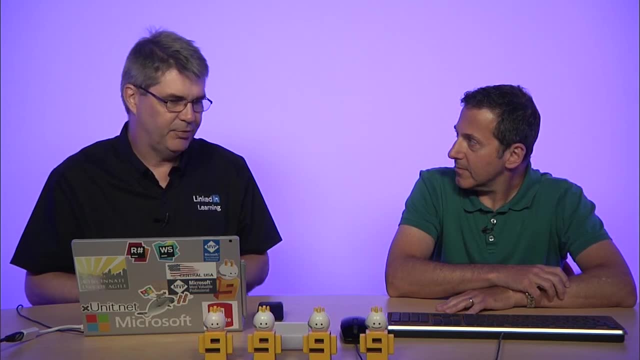 really the one I like better is provides an alternative to subclassing for extending functionality. So let's talk about Starbucks. Okay, Right, I typically only get one thing when I get to Starbucks, but I know that they have probably 2,000 different variations between the syrups. 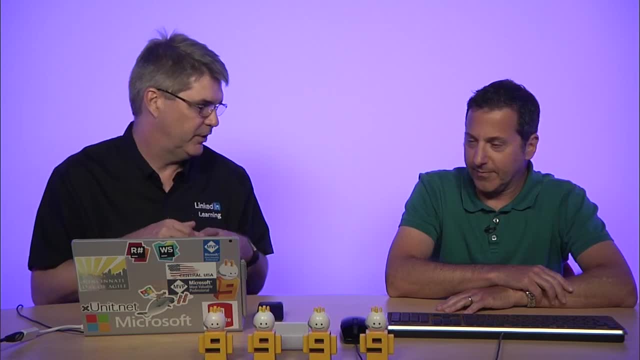 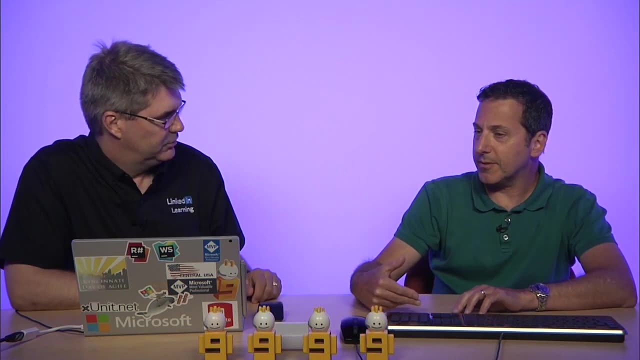 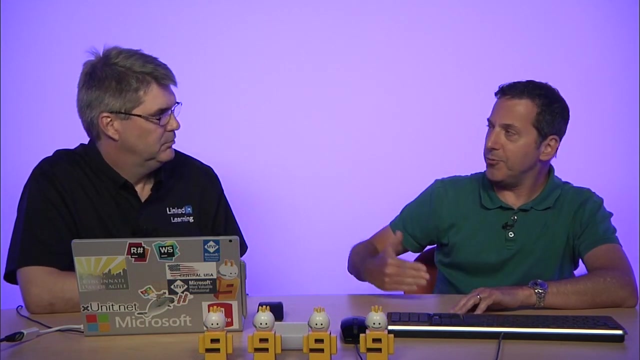 and the size, and the extra shots, and soy milk versus regular milk. Everything you ask for is another attribute of that cup of coffee. It's another cost. So what you would hopefully not do is have a new class for every single possible permutation of a cup of coffee. 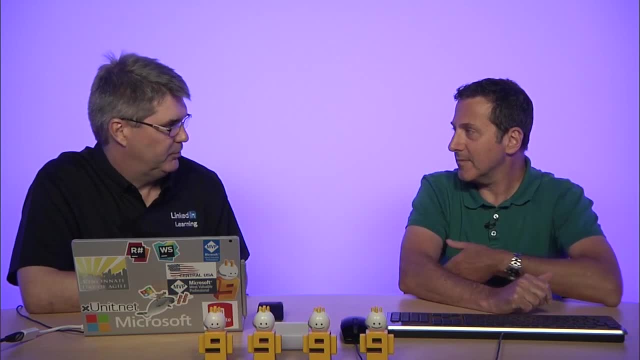 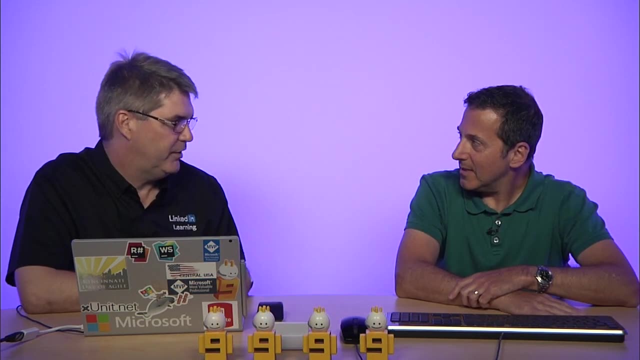 Right. The other terrible end of that spectrum is a really big if statement- Yeah, Which I've seen. but if we want to be object-oriented, then we might say: well, we should create a coffee class and a coffee with creamer class. 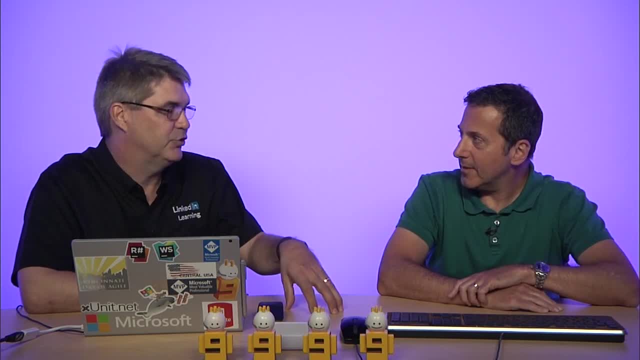 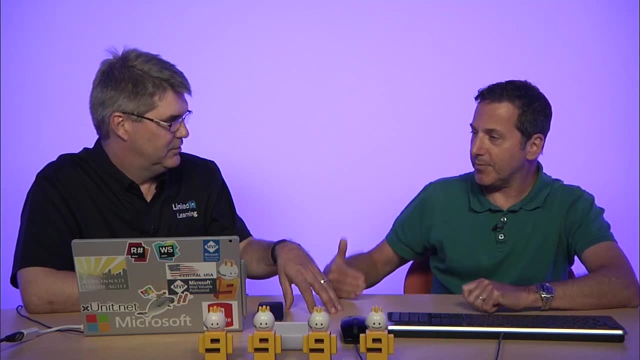 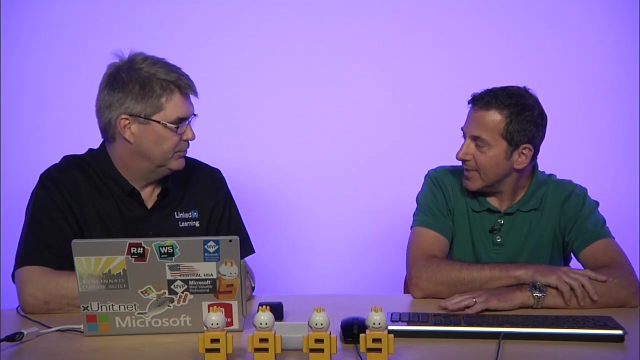 and a coffee with an extra shot of espresso class And a class with two shots of espresso Right And creamer and espresso and two shots of espresso in a particular temperature. And if you think about all the permutations, And we have just imploded on ourselves. 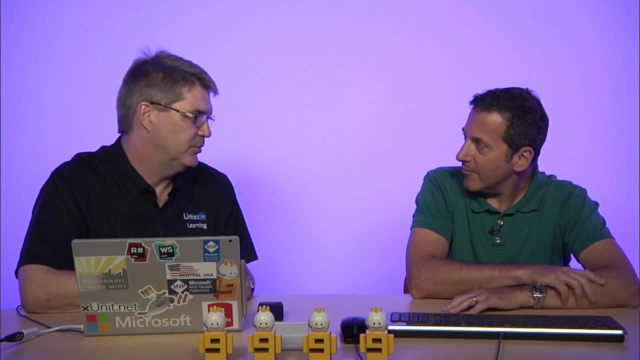 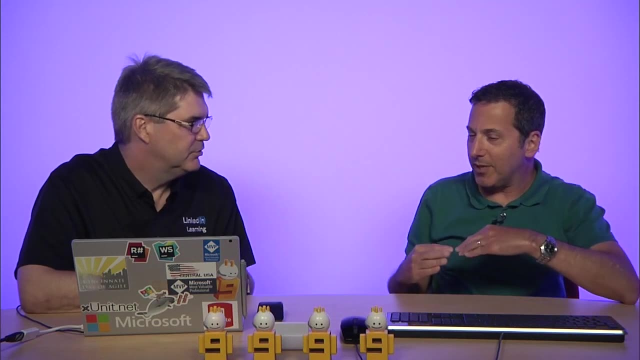 Yes, We'll never be able to support this code and probably never get it shipped Right. Or you could create a class with 2,000 properties That mostly never get used, Of which in any given cup of coffee you might be using two or three of them. 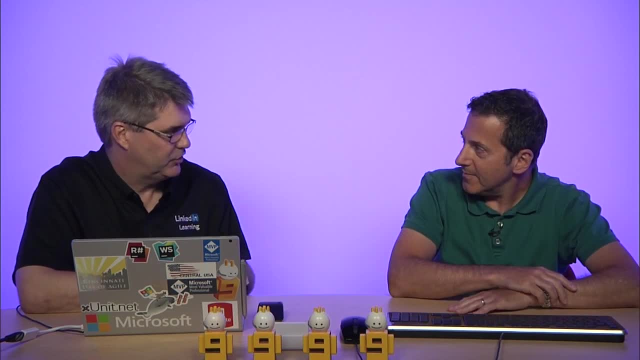 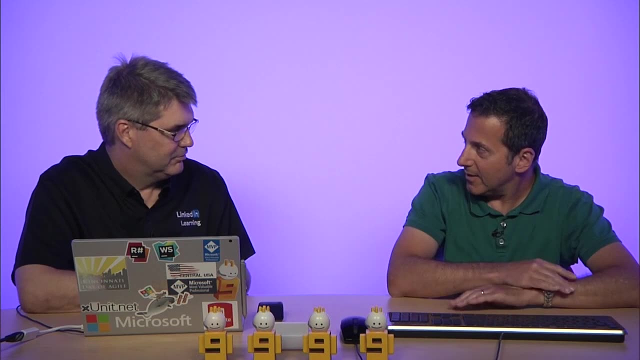 Right, That seems kind of wasteful. And then you still have to have a big if statement to figure out how much it costs, Right, Or a for loop to loop through every property. Yeah, And how do you know what the property names are? 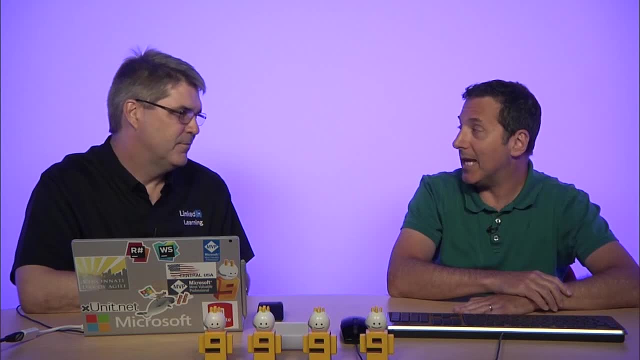 Are you using reflection to go through the class to find out what the property names are? There's got to be a better way. There is a better way, But before we get into the better way, let me talk about a real-life example where this would have saved me thousands of lines of code. 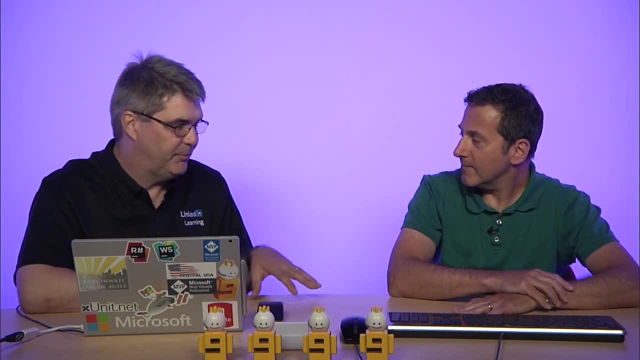 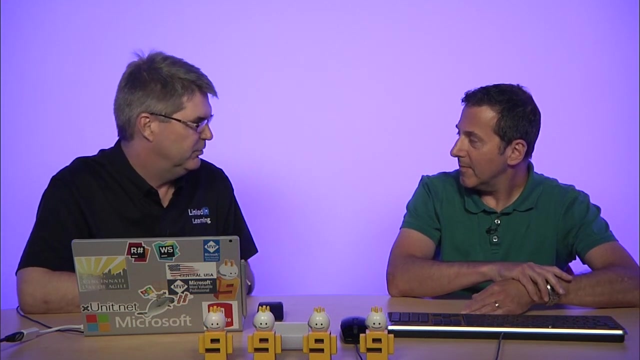 So I did a project on JavaScript in the early days, like right before. JavaScript was totally cool And it was a configurator for a high-end bicycle shop. So these are Tour de France style bicycles, right? Not the I'm going to go ride around Seattle bicycles. 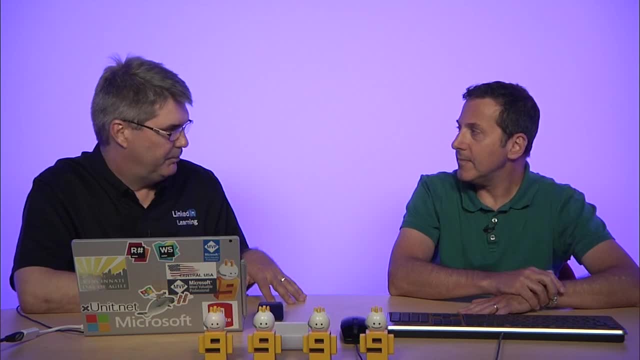 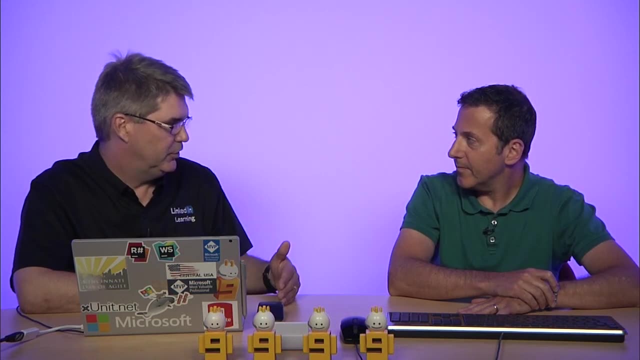 And this is all in JavaScript. It was all client side And based, for example, based on what frame you picked, you had to get wheels, But the wheels were limited to. you know, based on the frame And then based on what wheels you picked, there were brakes and brake shoes and all the parts of a bike. 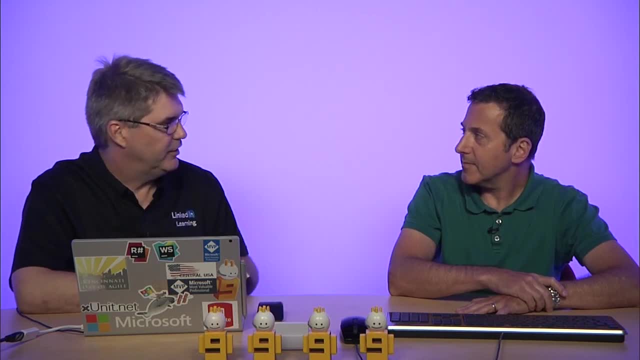 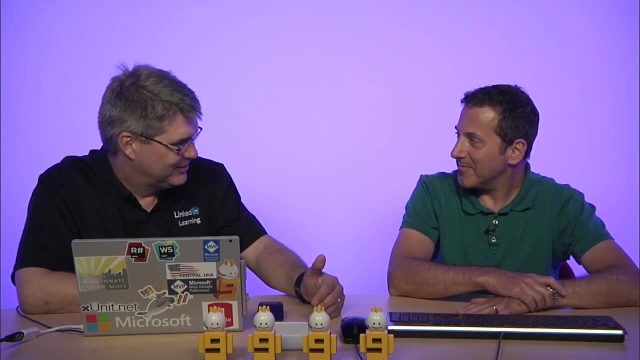 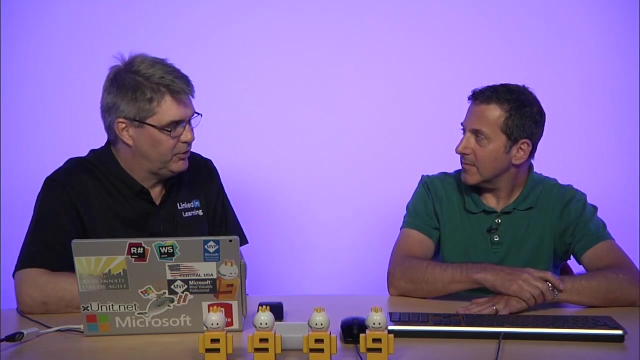 I mean literally rebuilding these bikes was crap. Yes, Guess how I wrote that. A ginormous if statement Started at the top: If they selected this, then show these options. Yeah, And then continued on down the road And my name's still on that code. 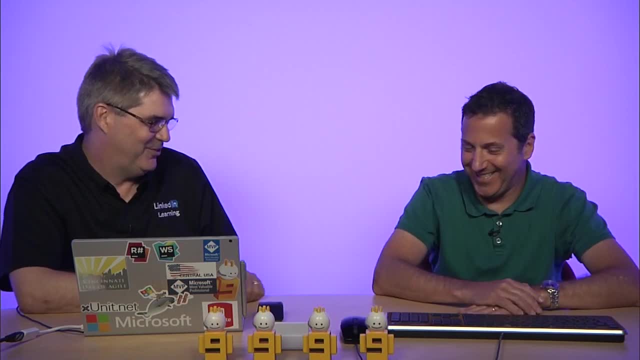 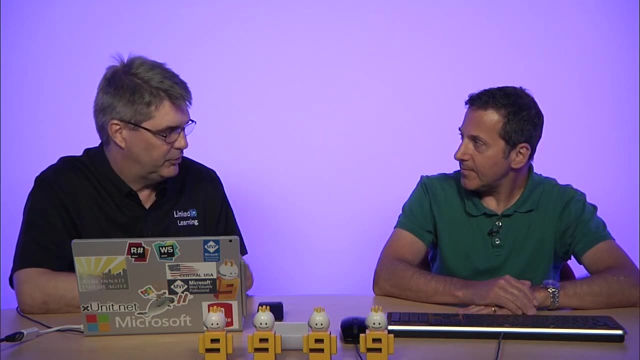 I've been trying- unsuccessfully- to have my name removed from the code, So I don't want to take blame for it. But it was before I knew the decorator pattern- And this is, you know, many, many years ago- And once I started doing some really deep research into patterns. 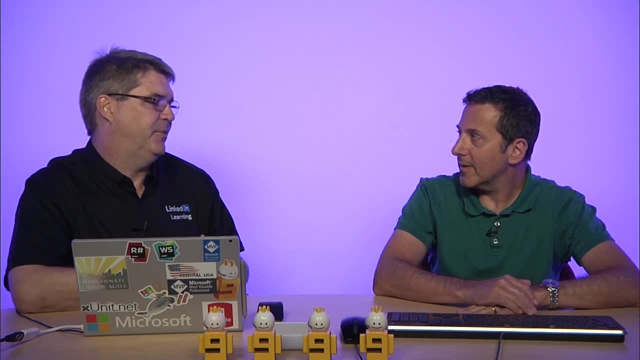 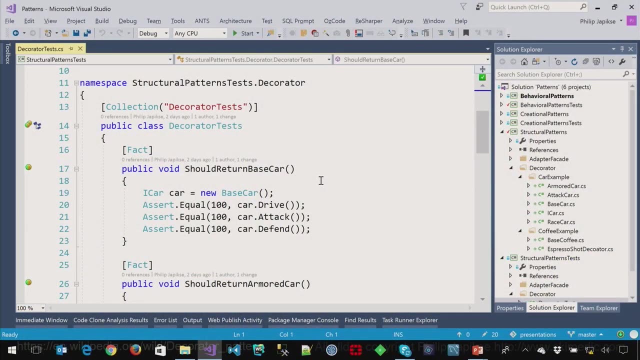 I saw a decorator and I went: oh, I've got to save myself so much time by building that configurator, So let's talk about how the pattern works. Okay, So we've said this on every episode. I'll say it again, just in case you're jumping in now. Okay, So we've said this on every episode. I'll say it again, just in case you're jumping in now. Okay, So we've said this on every episode. I'll say it again, just in case you're jumping in now. 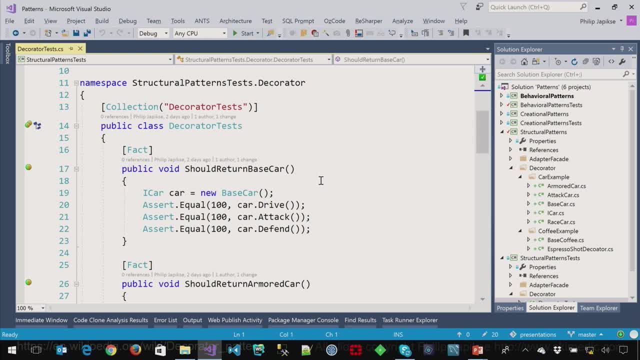 So we've said this on every episode. I'll say it again, just in case you're jumping in now. I tend not to use real-life examples in my sample code. I just want to use silly things so that we talk about the pattern. 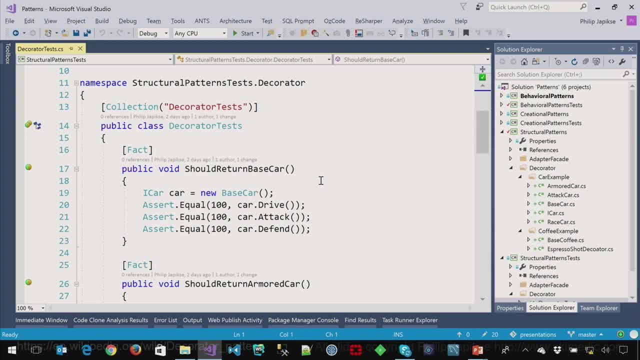 and not get hung up on banking or insurance or things like that. So I was watching Speed Racer the movie, which wasn't as good, as I remembered the show when I was a young kid, But they had different types of cars. 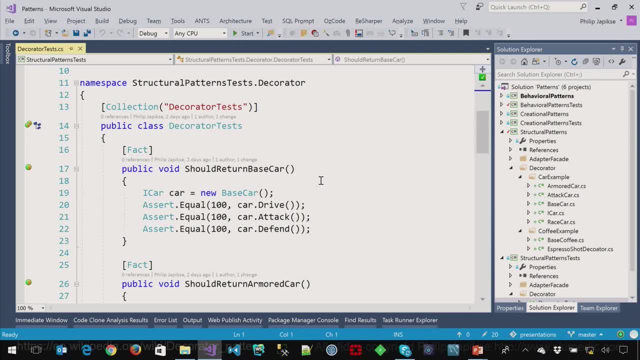 Yes, They had cars that focused on attack, cars that focused on defense. Of course, Speed Racer, the number eight, it was number eight, wasn't it? I think it was number eight. I think it was number eight. It was the fastest car around, right? 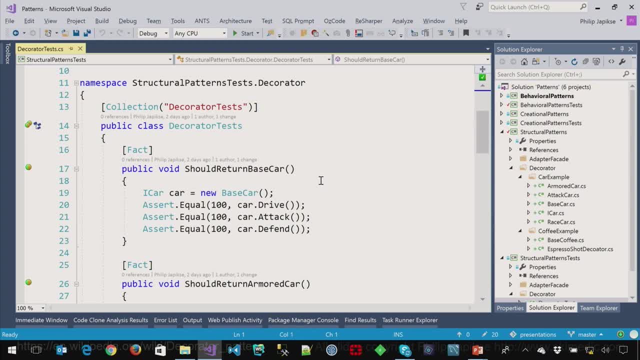 So I started thinking: how would I? What was it five, I don't remember, Okay. Well, I totally messed that up, didn't I Trying to bring in some pop culture, and I screwed up. So I started thinking about how would I program those set of cars? 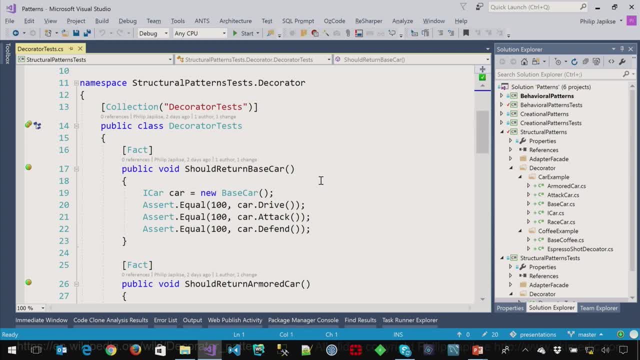 Well, I could certainly make a base car, I could make a race car, I could make an armored car and I could make an attack car. So I've got four cars And they're all cars, And they're all cars. 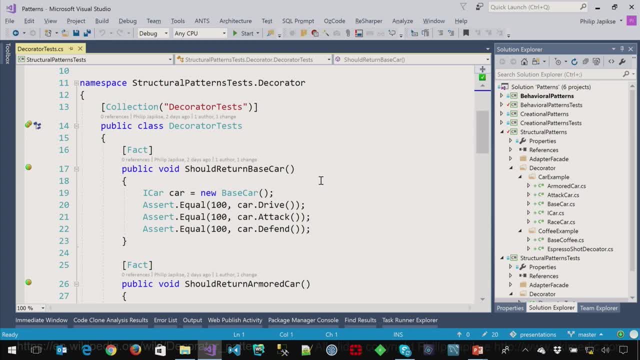 What if I wanted to put? What if I wanted to put guns on something with armor? Now I have a fifth car. I have the armored attack car. Now I want to soup it up. I have the armored attack race car. 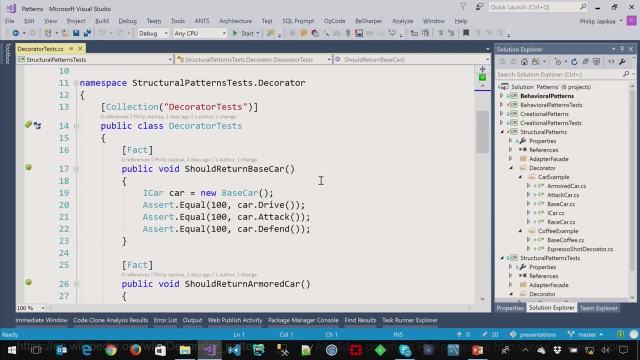 Now I have six classes, right, Yeah, You see how this gets exponentially worse, Very, very quickly. What we want to do is we want to decorate the car with attributes, Like you said. we could have a whole bunch of properties and start throwing values in there. 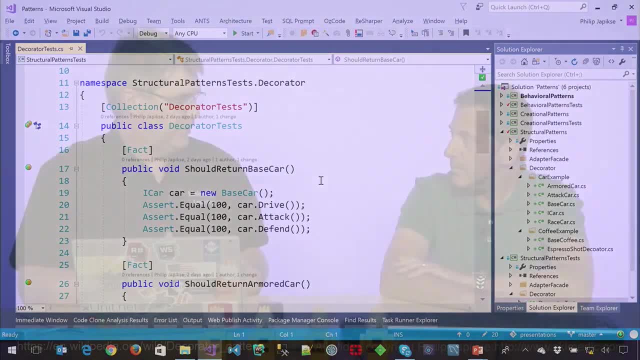 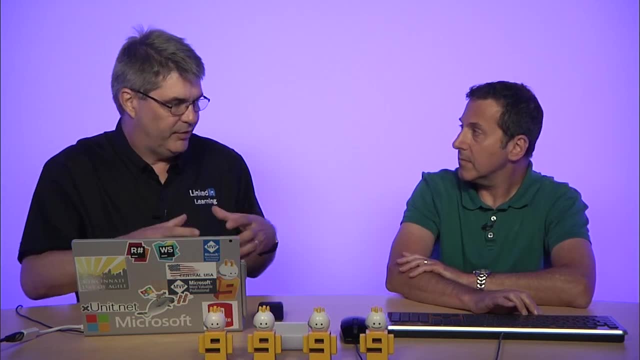 But then Losing that single responsibility. Right, I want the decorator for the armor, for example, to know what that does to a car. Okay, I don't want the base car to know what the armor does, because what if it changes? 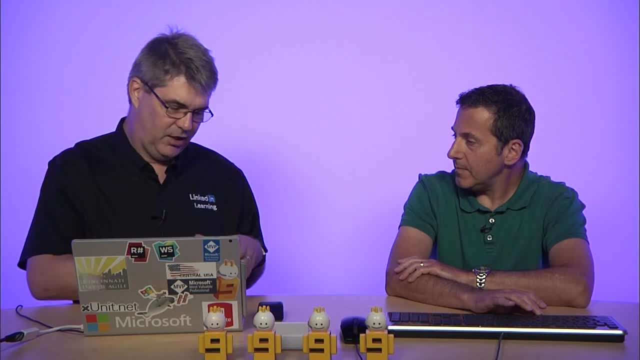 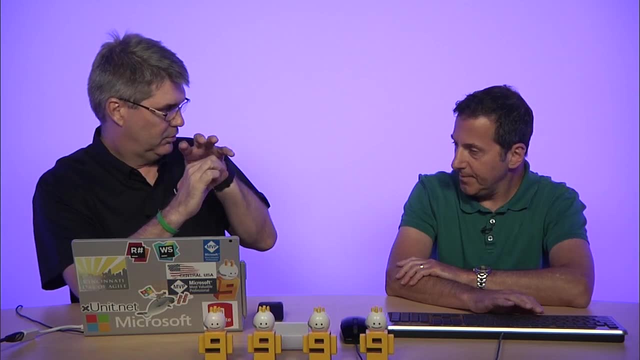 Right, Right. So we're going to imagine an onion where we have our car at the center and we're going to decorate that with armor. Okay, Decorate that with guns, Decorate it with a faster engine, Mm-hmm. 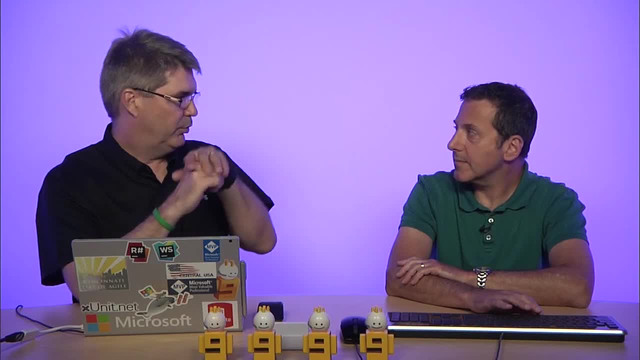 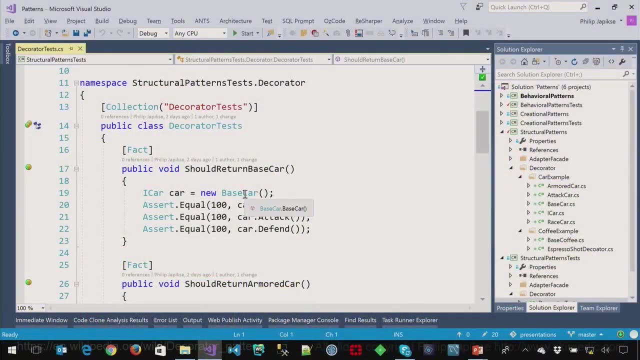 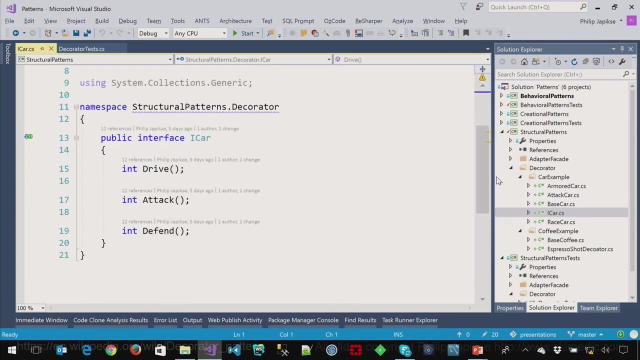 If you so desire, decorate it again with armor. Okay, So what we're talking about is basically building up this onion with decorators. Yep, So how does a decorator look? Well, let's talk about the I-car first. It just has three properties or three methods: drive, attack and defend. 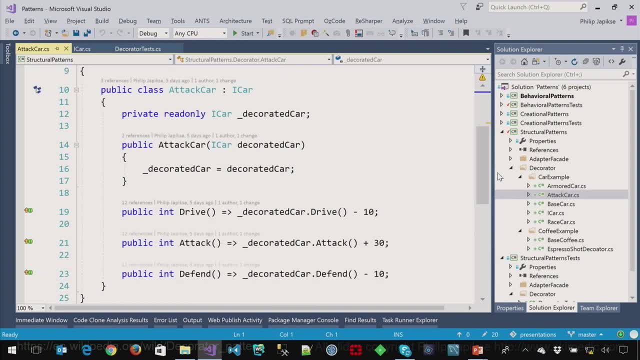 Let's make an attack car. So notice that an attack car also derives from I-car Yep, Because it's a car, Because it's a car, It gets passed into its constructor, an I-car. So this is a perfect example of why we want to program to an interface. 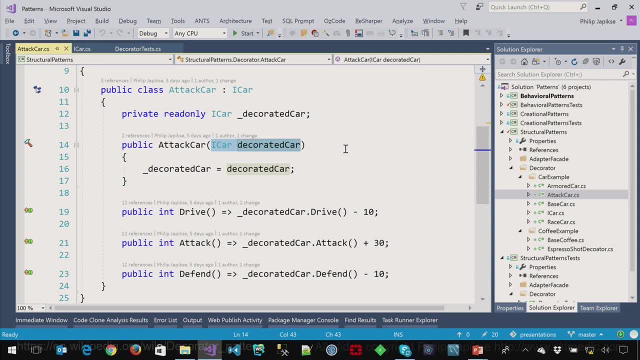 because we don't know what kind of car it is. We just know it's a car. Mm-hmm, If I was programming to an attack car then I could only pass in an attack car or an armored car. So we've opened up the possibilities by just having the interface there. 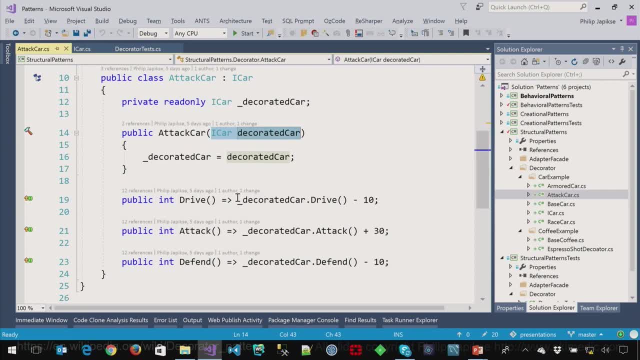 Mm-hmm. The attack car knows, Mm-hmm, That the drive, the speed, gets diminished a little bit, So it doesn't matter what the value was Mm-hmm. Technically these parties should be properties, but whatever. 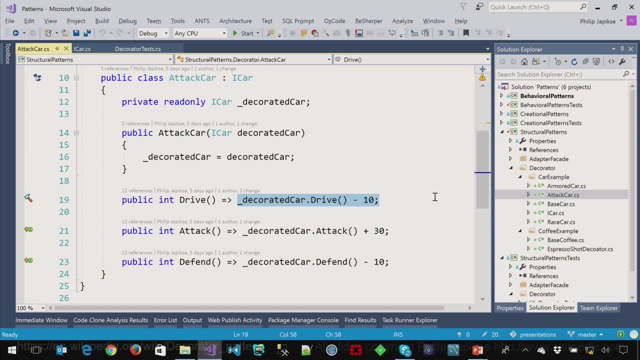 Again, it's demo code. The attack vector goes up significantly and the defend drops Okay, So I've encapsulated the entire logic of what an attack decorator does in the attack decorator, So nothing outside of the attack decorator needs to know. 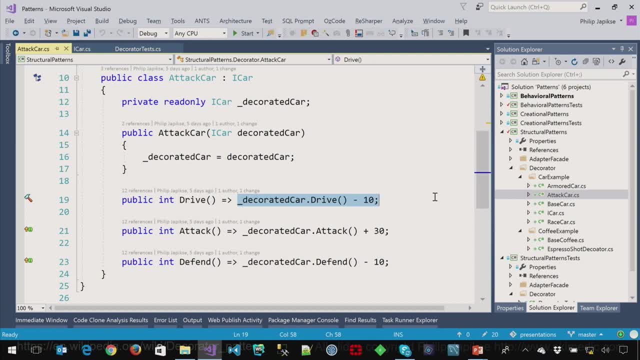 Okay, If I change it later and say: you know what? We are able to have lighter weight guns for the next race across the desert, then maybe the drive doesn't go down And I only have to change it in one place. I've encapsulated that logic. 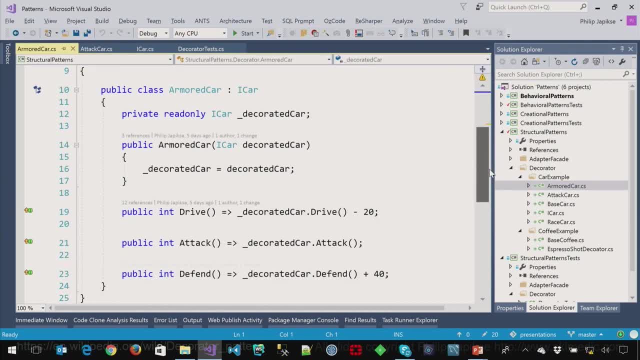 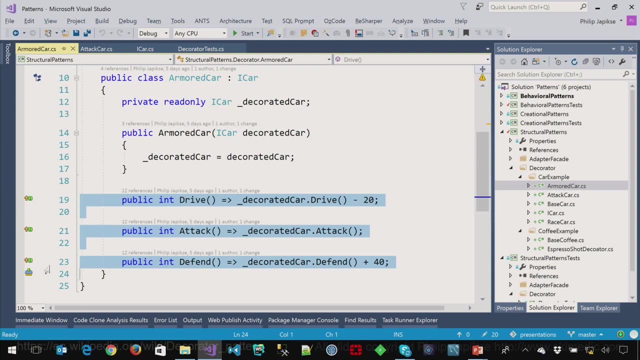 So let's say we want to put armor around that. We then pass that decorated car, just an I-car- into the armored car decorator and it then modifies The attributes And then if you defend it again, you could pass that in again. 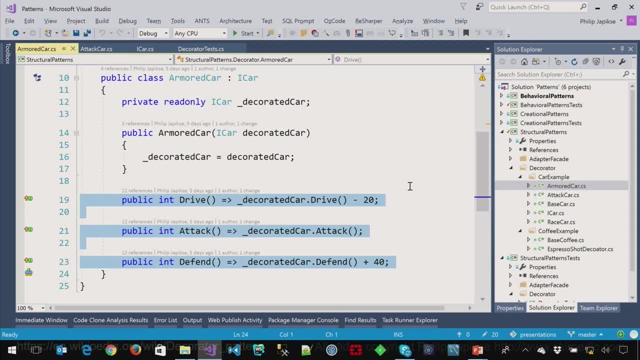 and it would decrement the drive and increment the defend again, Right, Okay, So I could have as many combinations of armor and guns and speed with only having those four classes. Okay, Let's say we come up with something new: the flying car. 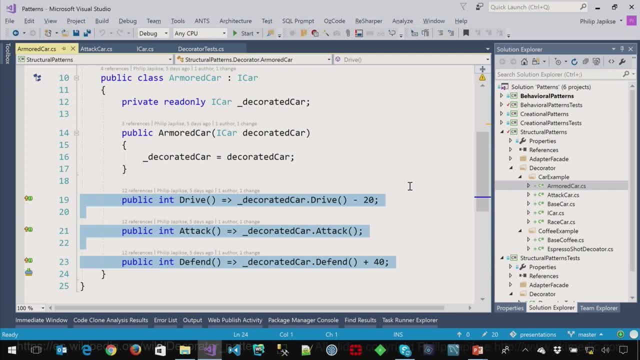 Right, It has a jet pack and wings or something. Well, instead of having to now look at each of these individual cars and say, well, what would flying do to it? we just make a fly decorator and we figure out how that affects the attributes of this car and we're done. 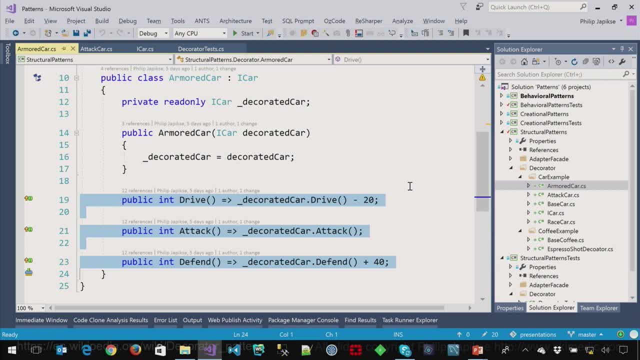 We've added one class and we've added a, basically you know n factorial number of options. So in this example, each of the cars implements I-car. that has the same methods and properties. Yes, And you're incrementing or decrementing the drive, the attack, the defend. 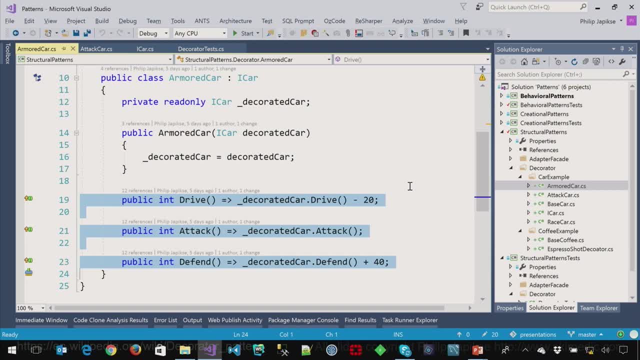 So couldn't you just change properties? You can. The problem with changing, just changing the properties. and we'll look at the coffee example next, because I think everybody watching this show is probably a heavy coffee drinker. anyway, Excuse me, 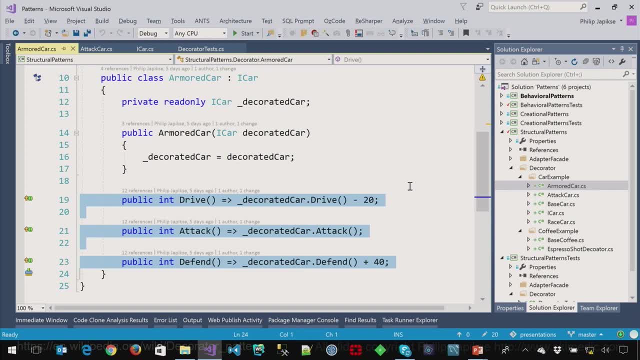 Well, to get through the series, you've probably been a lot of coffee drunk, Or a lot of drunk coffee, Pardon me. All right, So I could just change the properties outside of this decorator, but then the problem is, I lose the encapsulation. 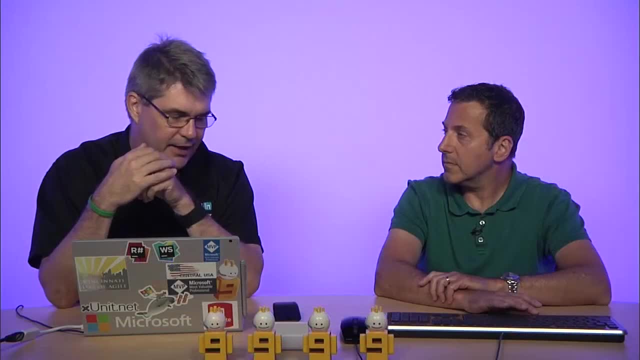 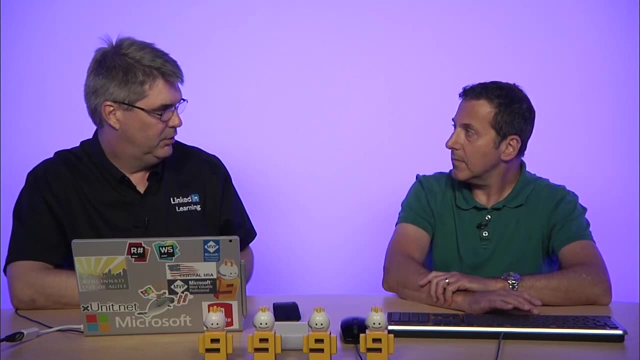 Every time I want to add armor to a car, I am then having to remember what that does to the properties. Okay, If I would then want to go remember the simple factory. Yep, If I want to go and add a new type of car. 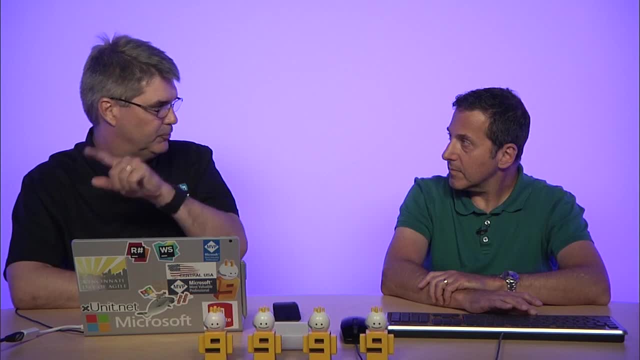 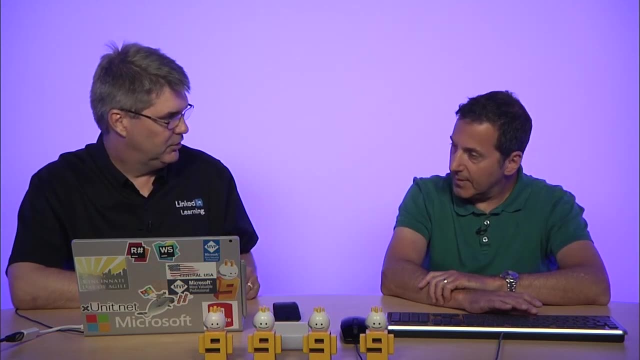 now I have to go to every place in the code where I've updated the car's properties to make sure that I'm taking into account that new type of car. Okay, So this is all about encapsulation, Got it? But also extending a class while modifying it. 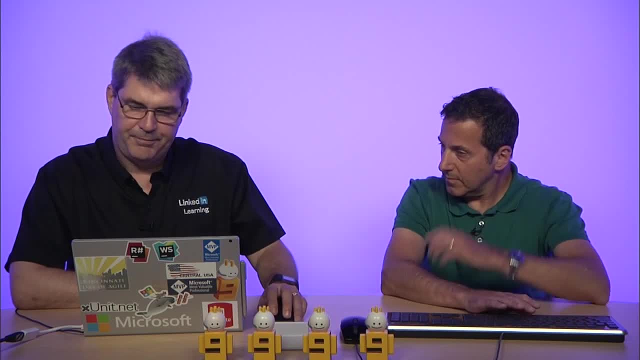 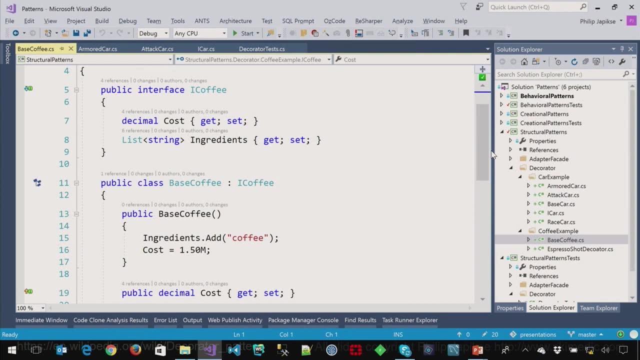 Okay, All right. So let's look at coffee. Everybody understands coffee, So we have cost and we have ingredients, Mm-hmm. So we'll start with the base coffee having a cost of $1.50 and the ingredients is just coffee. 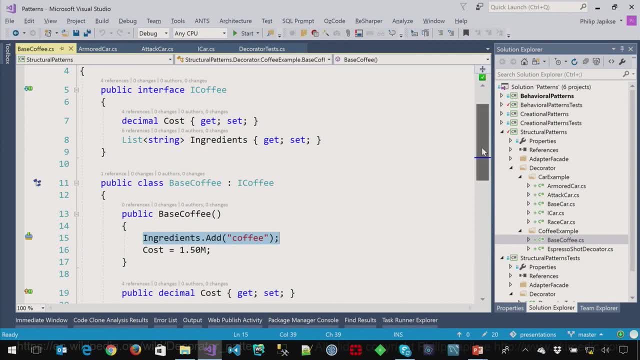 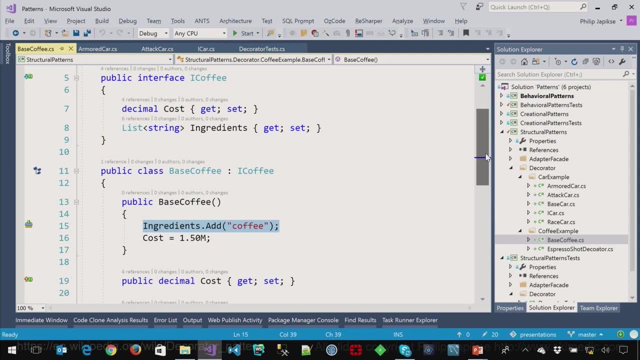 So here we're going to get around the issue of having a single class with thousands of properties, or thousands of classes which are all coffees, but they vary in various ways. Yes, Okay. So here we have a list of ingredients, right, and the cost. 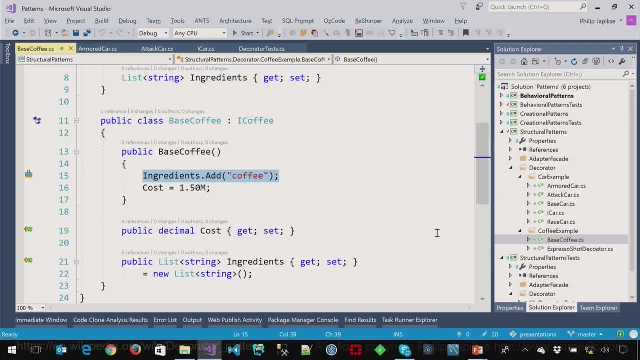 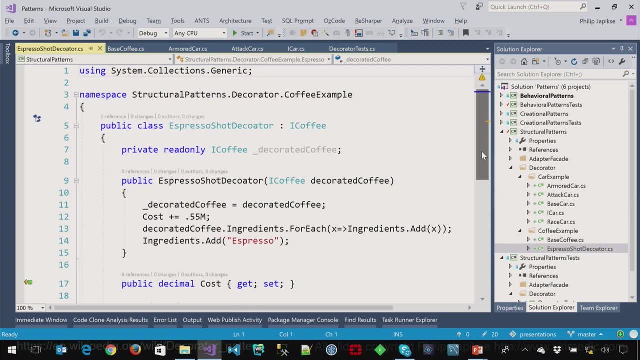 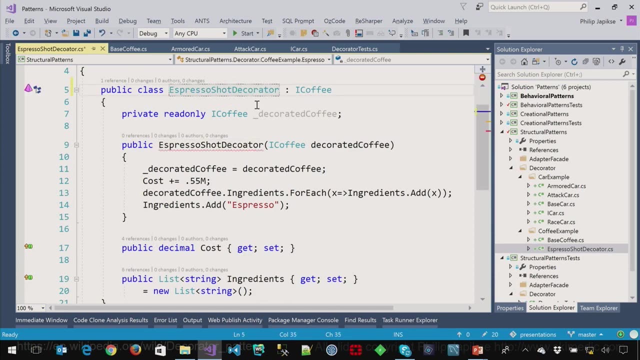 Okay, Set that in the constructor. Now we're going to add a shot of espresso. Okay, So we have this espresso shot decorator, Or decorator, Or decorator. You know what, Through the magic of TV, we can fix that just like that. 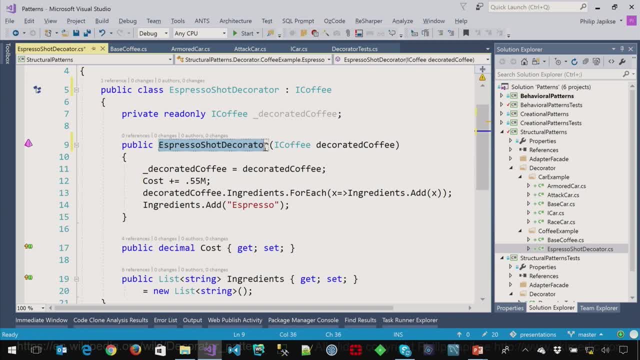 There we go And we have our constructor which takes an iCoffee Yep. We increment the cost Okay, By $0.55.. Mm-hmm, And we get all of the ingredients from the currently decorated car, Sorry. 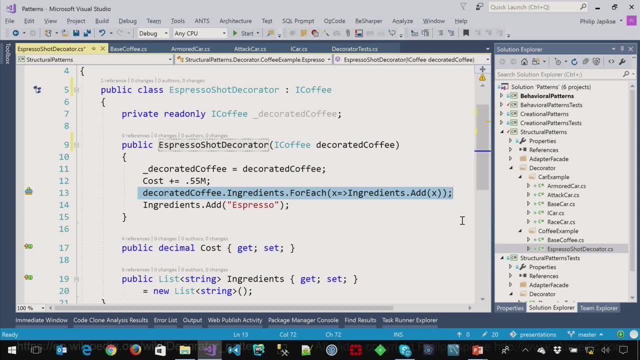 Coffee. So in the car mode, Coffee Yep, And then add espresso to it. Okay, Now, if I wanted to have a double shot of espresso, You would just run that again. I just run it again. And this is not a complete implementation, because you know, obviously, if you're making 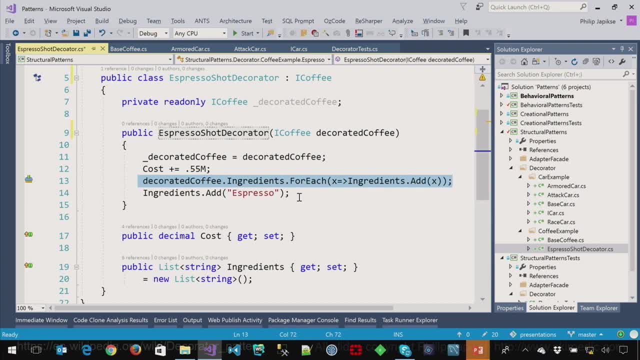 a coffee, you're going to have to somehow generate all the ingredients and the right ratios and things like that. But what I'm trying to show is just how the decorator will decorate those base classes: Mm-hmm, Or not the base, but the past-in interface. 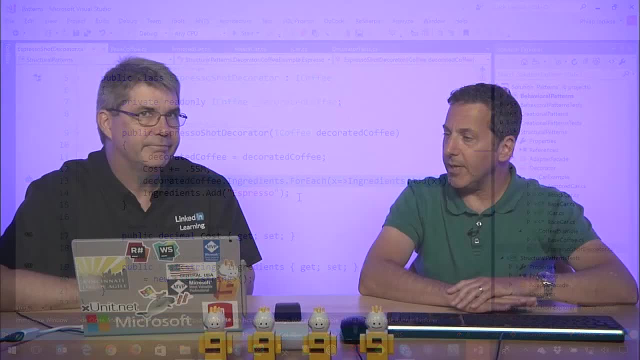 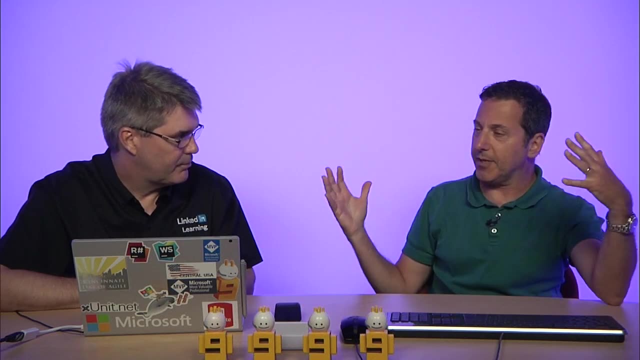 Right, And build it up And you might. you would wind up with a decorator for everything you can do to this coffee, right? Yes, So you're still going to have a very long list of something, Right? But they're all encapsulated and easy to work with. 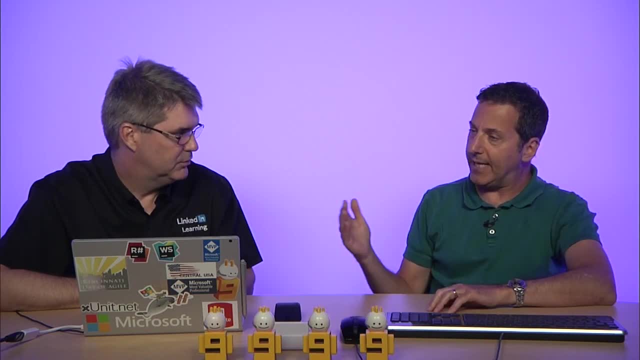 And then to add something to the car that you're going to need- you're going to need a lot of things, Right? So you're going to need a lot of things, Right? And then to add something to the car: the coffee, the superhero, whatever it is you. 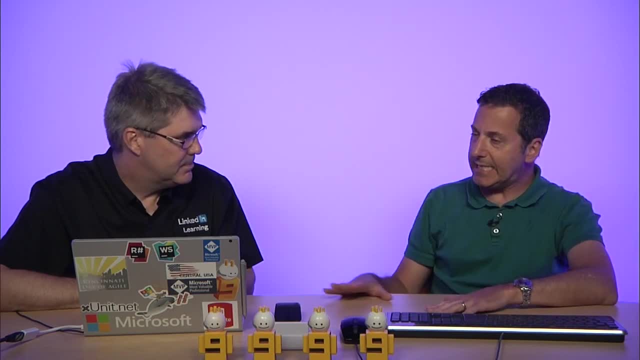 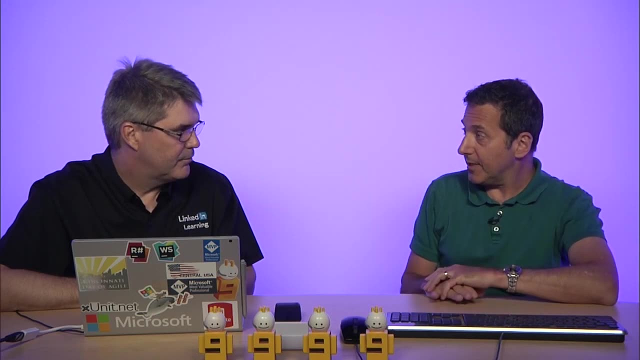 just call the decorator. Yeah, So it's much easier to manipulate the object and add things to it or potentially remove, Right, I assume you could do. you could use decorators to take things out. Yes, Yeah, It's really not part of the pattern, but I don't see why not. 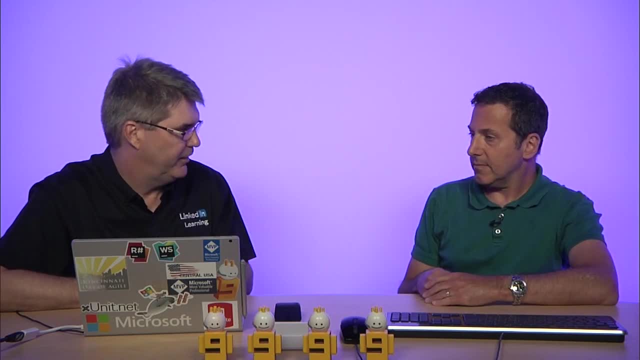 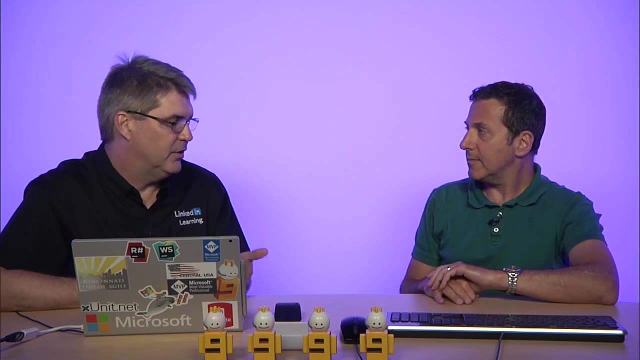 I mean, obviously you would have to modify, like in our example here: modify the ingredients list, Right. Might use a memento pattern, Yeah, And then add things into a specific state, Right. But you know, you were talking about having to have all these classes for all the things. 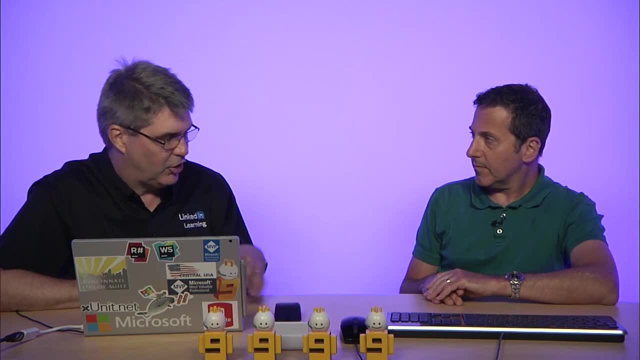 you can do, which is true, You know, in the car example, we only had four classes. In this particular coffee example, all we can do is add espresso to it, If you're at a Starbucks or you know some other coffee place of your choice there probably. 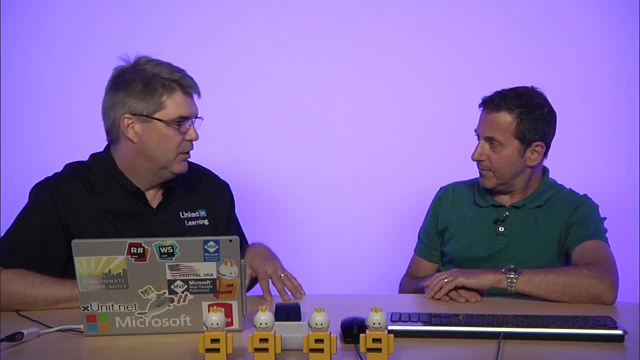 are well over 100 options. you can do to a cup of coffee, but you're only writing one decorator for each option, Mm-hmm, As opposed to writing a class for each combination of options. Right, Right, Right, If somebody comes and orders a half-caff, double decaf, soy latte with cinnamon and 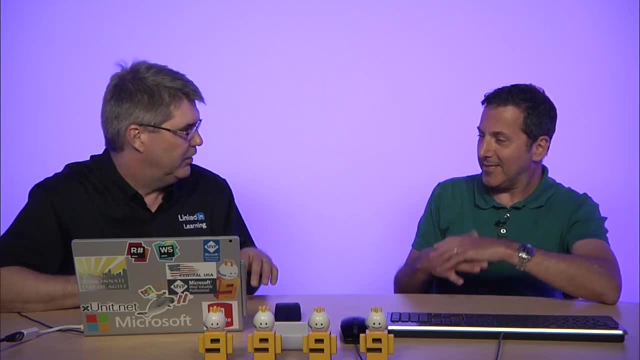 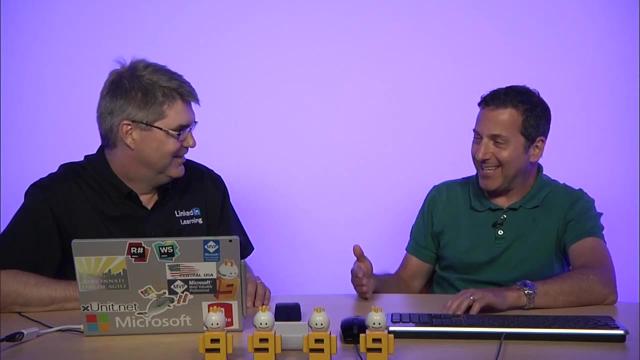 chocolate. I don't even know if that's a thing, but you know, Here's now. Yeah, How do you build that class Right? You don't? You don't? It's a cup of coffee, Right. At the end of the day, it's a coffee. 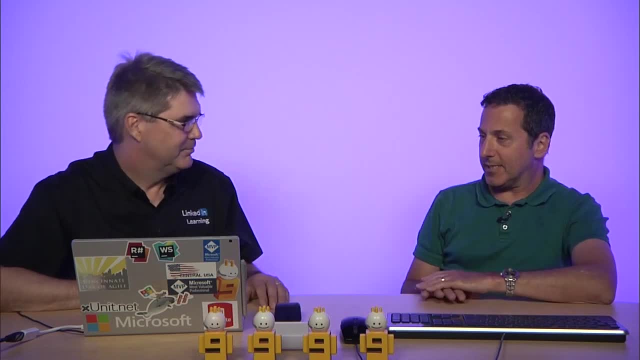 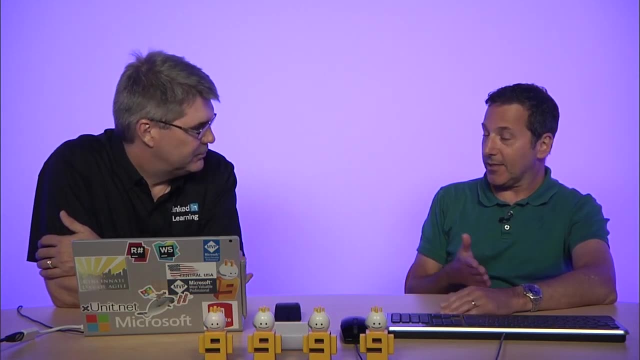 Yeah Right, And I've added soy milk to it. It's a coffee with different attributes. Yeah Right, It's easier to adjust the attributes and end up with a coffee. Yes, Because the coffee has cost. Right, It has ingredients. 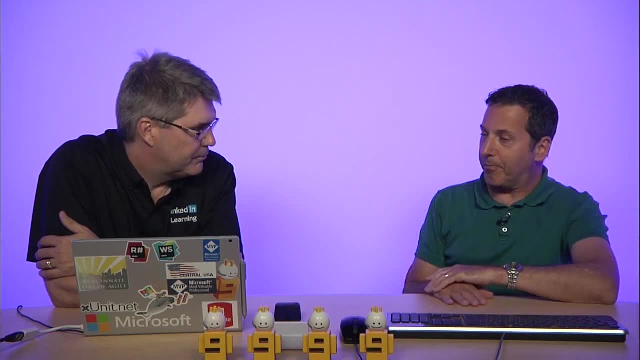 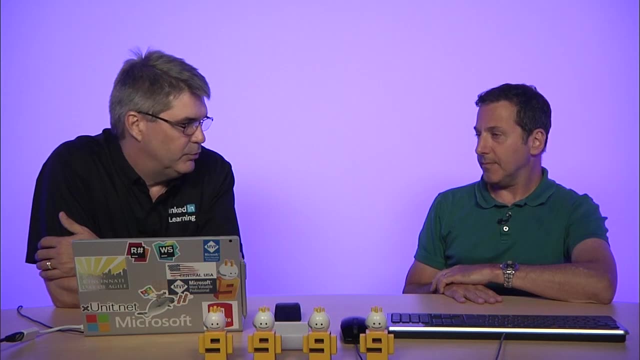 Presumably It has ingredients. Yep, Right, There are basic elements that a coffee has And instead of having some god class- Right, You know that knows what all these things do- Mm-hmm And then potentially have repeated code and other problems. 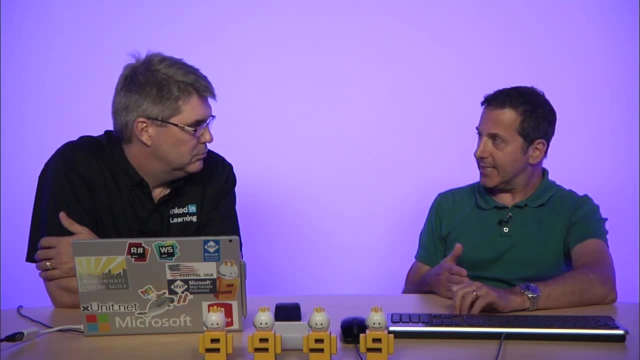 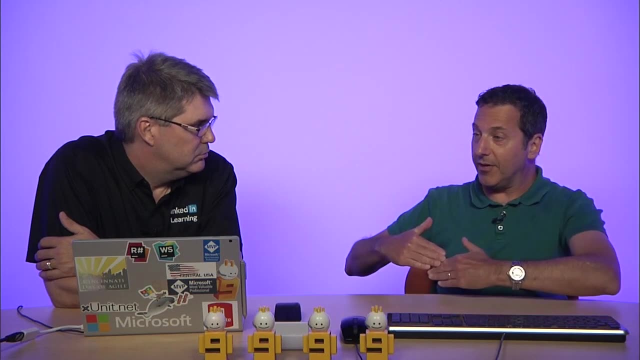 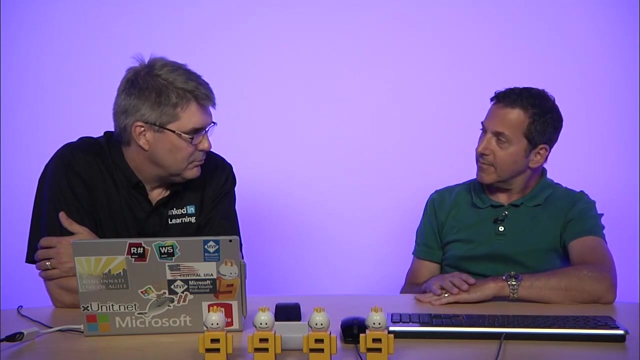 Done, Done Right, And you also wind up with very efficient instances, because, instead of having a coffee that has that, doesn't have 997 things and has three things, you've got a coffee that has three things. Yes, Cool Yeah. 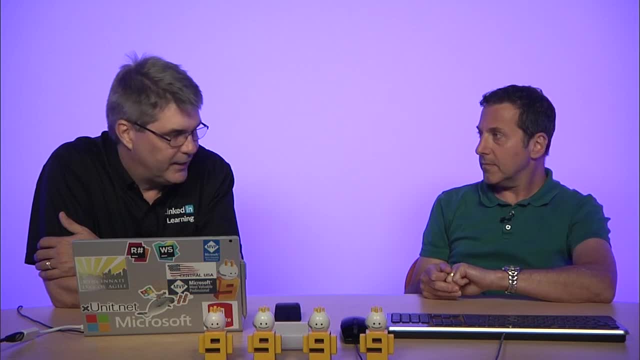 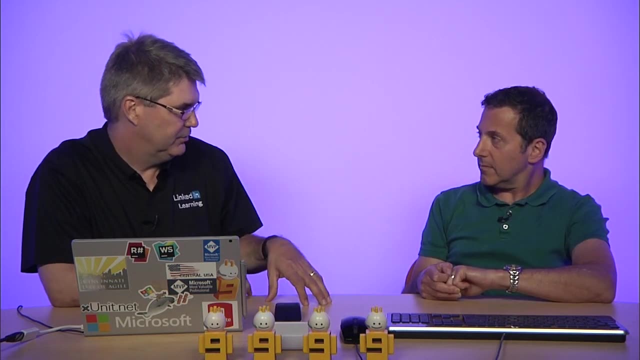 That's nice And I think that's a great example for the bicycle system Mm-hmm. Had I known about this pattern, that could have been so much easier, because I would literally start with a bike, an iBike class. 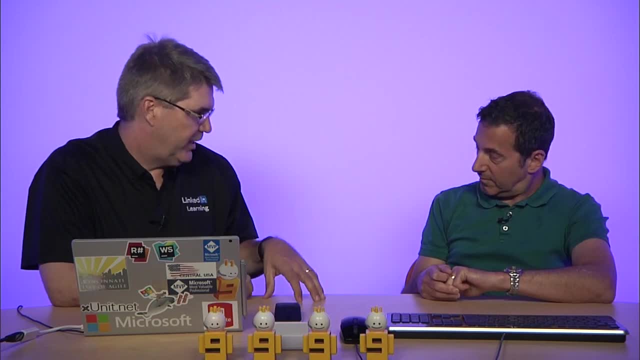 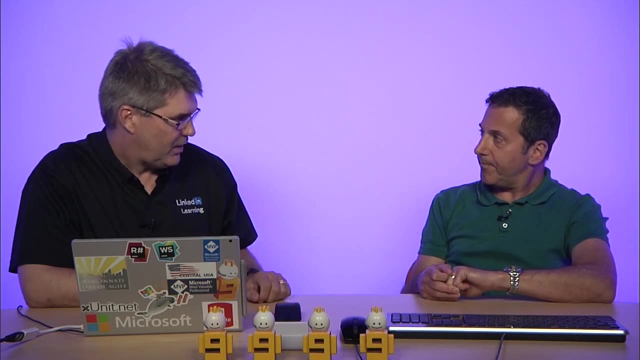 Right, Yep, And ingredients would be frame tires, brakes, gears, Yeah, That type of stuff, And then just building up the cost as I go. Yep, There's still some additional logic you'll have to do, Like, for example, maybe you can't mix. 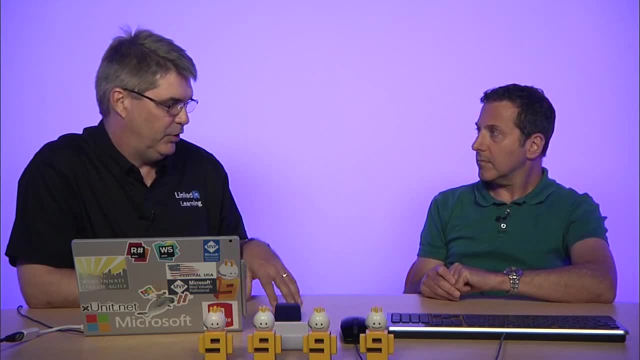 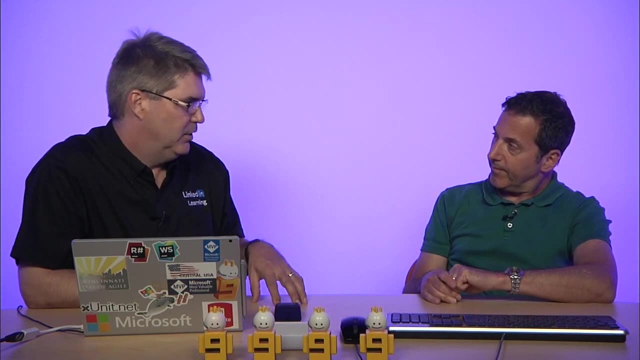 Going back to the car example, Maybe you can't put a race car in a car, Right, That's a good example. Maybe you can put a race car and an armored car together, Mm-hmm. Right. So that's outside the pattern, but those are things that might happen. 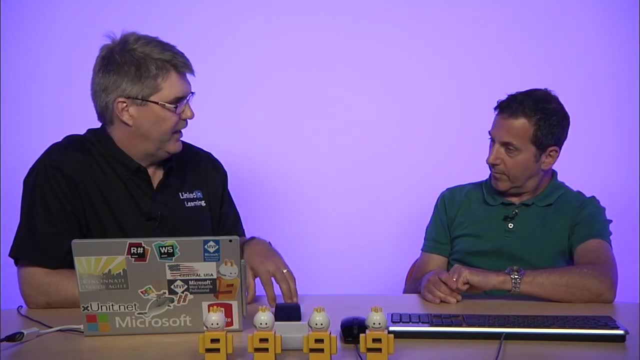 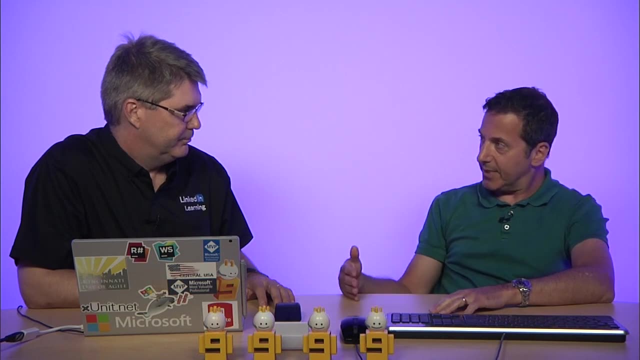 But you could certainly have a check saying: you know, if I can cast this to an armored car, then throw an exception or something like that. Sure, Sure, Yep, And it makes it easy to add new subsystems, Mm-hmm. 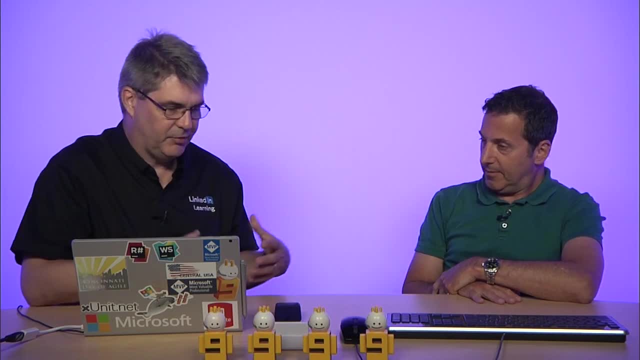 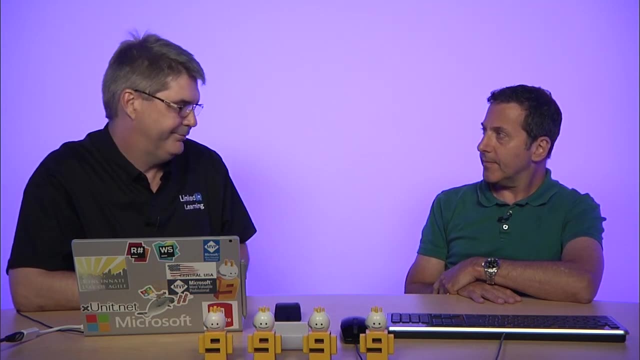 New collections of things, whether it's to the bike or the car or the coffee or whatever, Yeah, And you just keep decorating it and building it up to where you need to be And you've got a very small set of classes that have. 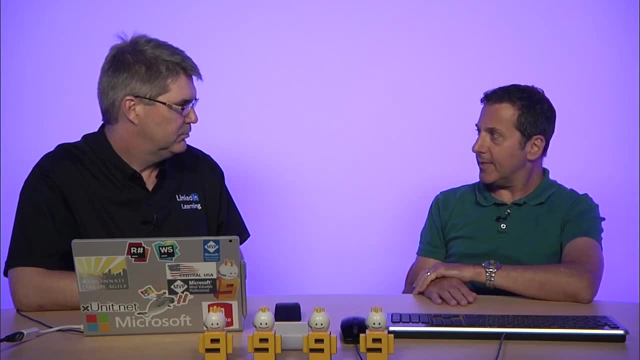 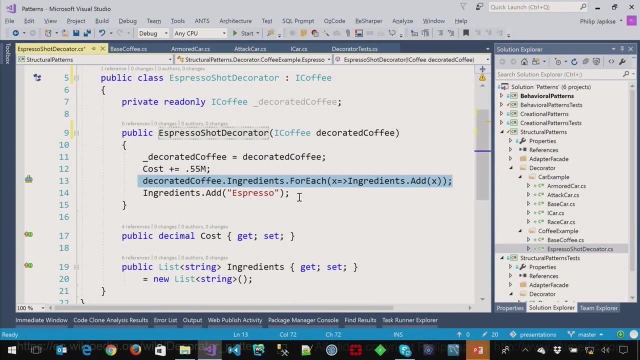 Yeah, Infinite capabilities of mixing and matching. Yep, Cool, Very nice. So, And that's the decorator. Excellent, Oops, We're back on. Hold on. There we go, There we go. I'll figure this thing out eventually. 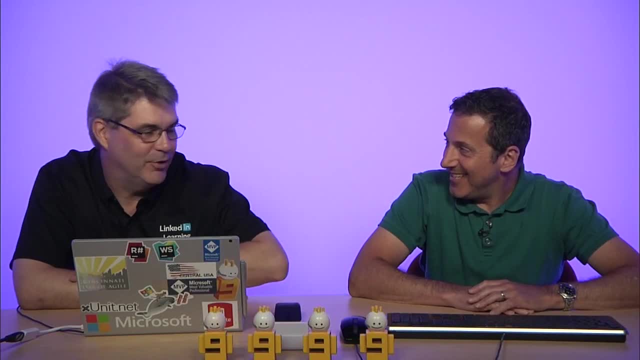 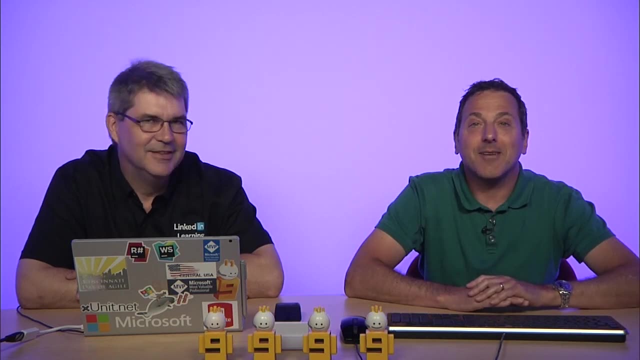 Like we said in the other episodes, today we're shooting in the B channel. Yes, So I'm in charge of switching back and forth, which is why it's not perfect. So that is our series on design patterns For now. For now. 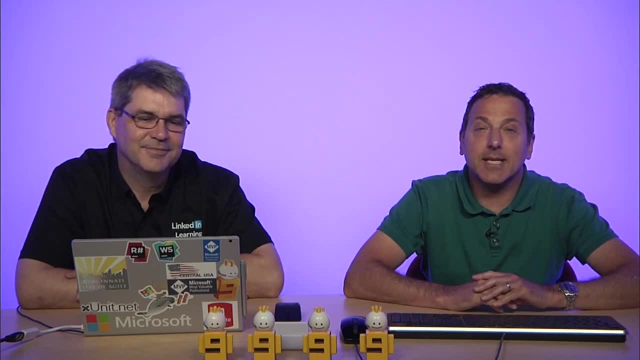 There'll be more. Yeah, Hope you enjoyed that, Really interested in your thoughts on this. I'm sure we've received them by now, but keep them coming And let us know what other types of things you'd like us to explore in episodes like.